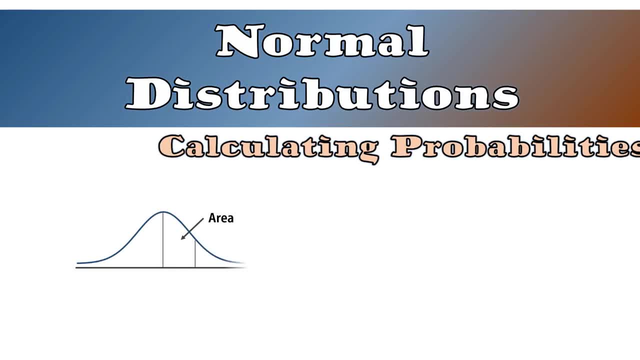 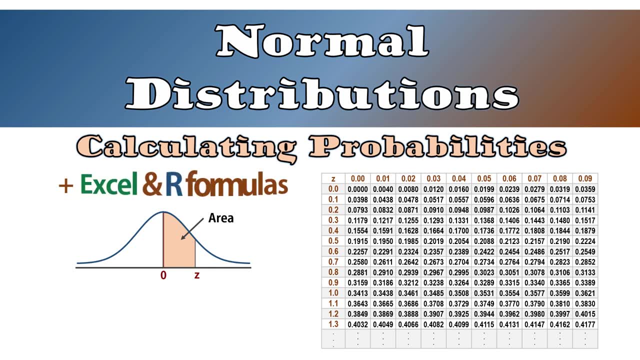 Welcome. In this video I'll be showing how to use the min to z standard normal tables to calculate normal distribution probabilities. I will also be showing software formulas along the way. Note that the table we'll be using in this video is the min to z table, That is, the areas provided in the table are 0 to z areas. 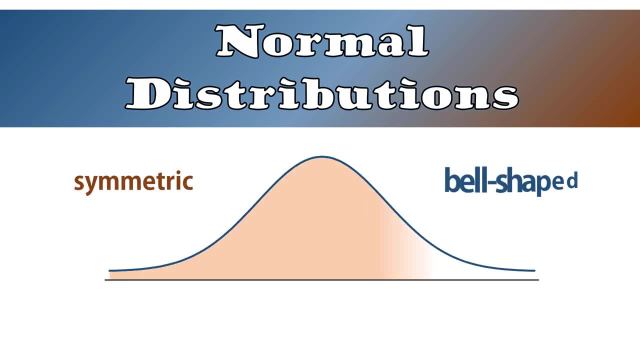 under the curve. A normal distribution is a symmetric bell-shaped distribution where the total area under the curve is 1 or 100%. Because it is symmetric, the min and median are equal and are at the center of the distribution. It means if we cut it in half, at the center. 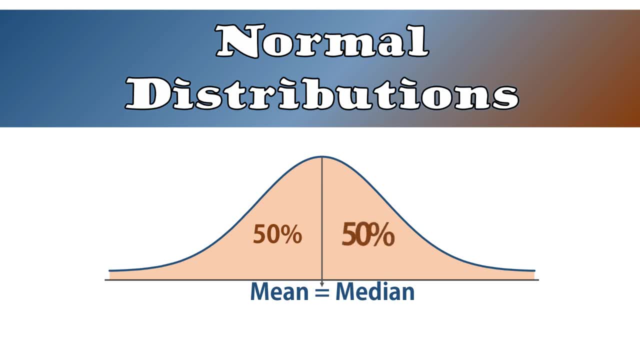 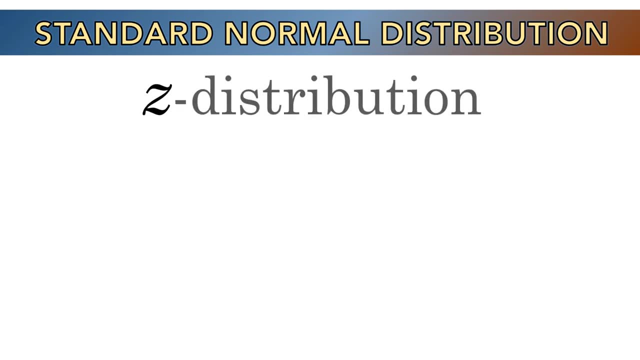 we will have 50% of the area below the min and 50% above the min. The standard normal distribution, or what is also called the z or z-distribution, is the standardized normal distribution with a min mu of 0 and a standard deviation of. 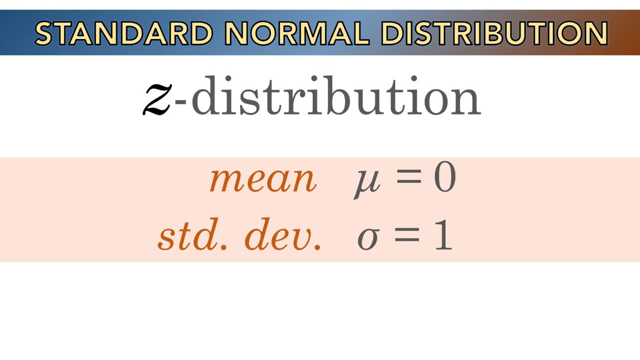 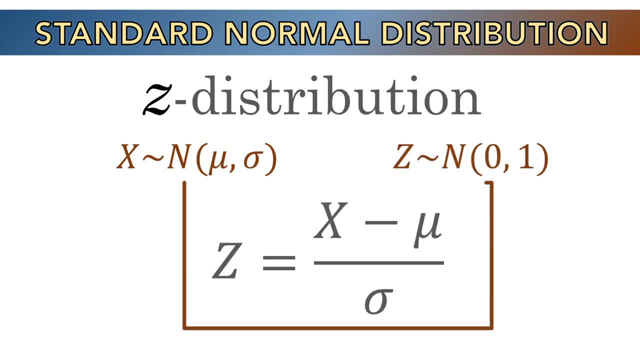 sigma of 1.. The formula for transforming a score or observation x from any normal distribution to a standard normal score is: z equals x minus min over standard deviation. The standard normal score, also known as the z-score or z-value, is the number of standard deviations. a score x is from the min. 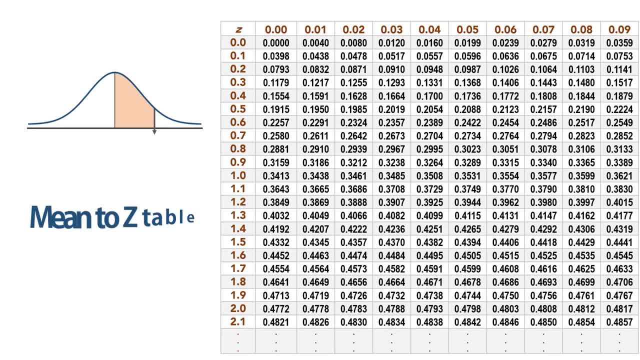 Again, the standard, normal tables we'll be using is the min to z table. This table contains areas or probabilities that are equal to or equal to, the number of standard deviations or probabilities from z equals 0 to the specified z-value as shaded under the curve here This: 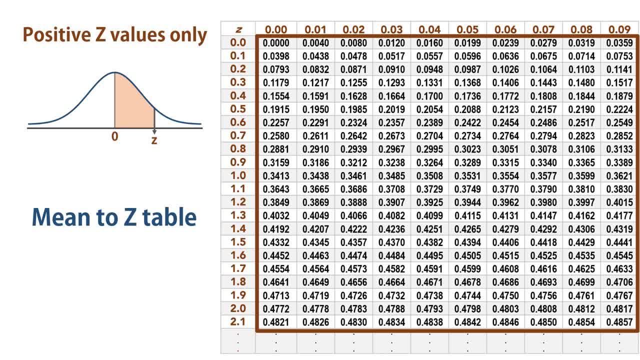 table comes in positive z-values only. To obtain areas for negative z-values we will use the same table and apply the symmetry property of the normal distribution In the first column. here we have the first decimal place of the z-score And at the top 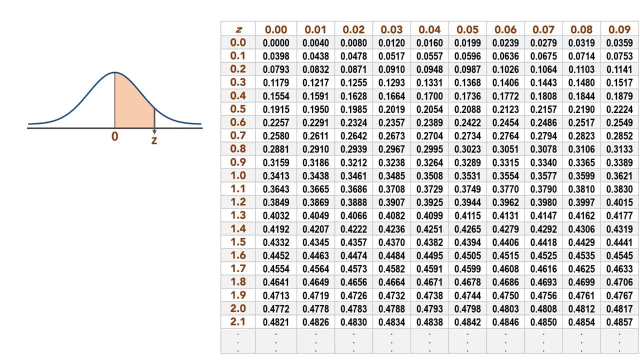 we have the second decimal place. For example, if we want the area between z equals 0 and z equals 1.32,, we will go to 1.3 in the row here and 0.02 in the column. So the area. 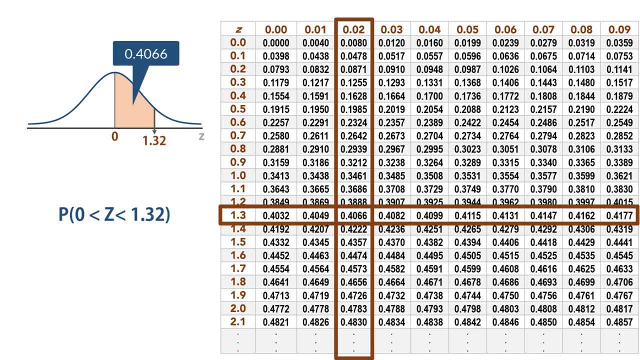 is 0.4066.. Now, because of symmetry, the area between z equals 0 and z equals negative, 1.32 will be found in the exact same way and it will also be 0.4066.. However, if we 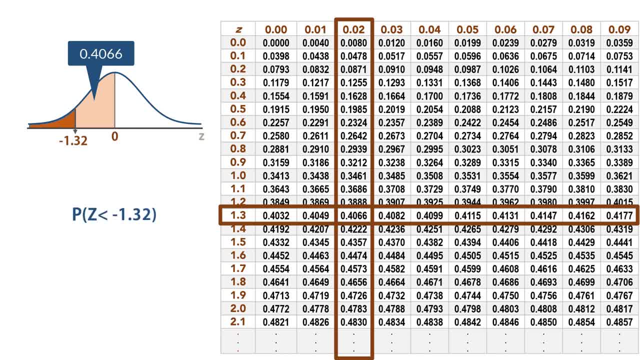 want the probability that z is less than negative 1.32, that is, the probability of this lower tail. we will use the same table and apply the symmetry property of the normal distribution. The area between z equals 0 and z equals negative 1.32 will be found in the exact same way. 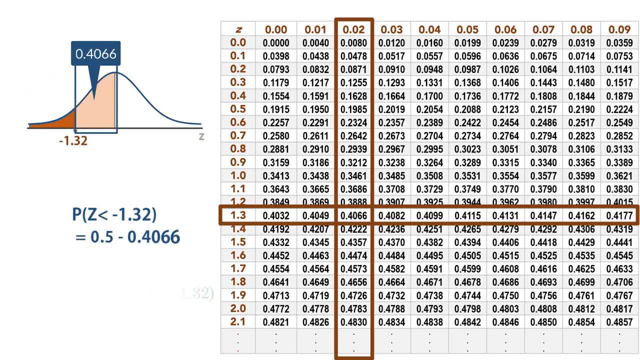 and it will also be 0.4066.. We will subtract this area from 0.5, since the total area below the mean is 0.5.. So this less than area will be 0.5 minus 0.4066, which gives 0.0934.. But 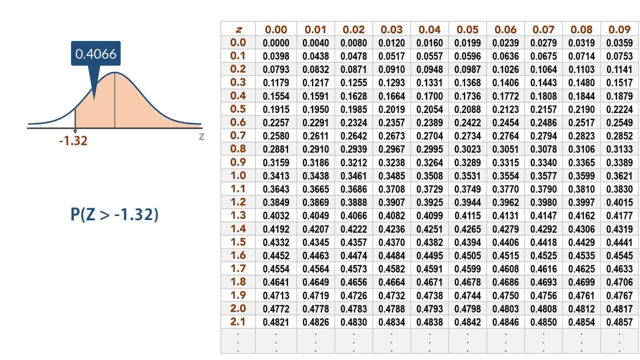 if we want the probability that z is greater than negative 1.32, we will add 0.5 to this area to obtain 0.9066.. Now note that the normal distribution is a continuous distribution, So there is no distinction between z greater than negative 1.32 and z greater than or equal to negative 1.32.. They 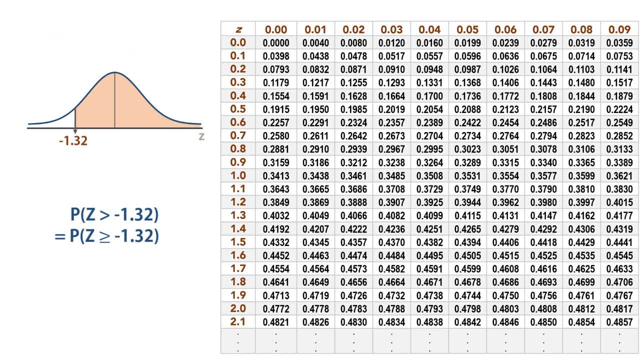 are treated the same way. Furthermore, if we want the probability that z is between negative 1.32 and positive 1.32, we will add the two areas or double the single area to obtain 0.8132.. Now let's consider further examples. Scores on a test are normally distributed. 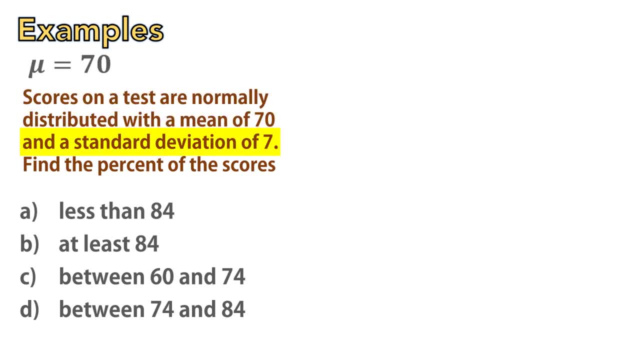 with a mean mu of 7.2.. So if we want the probability that z is between negative 1.32 and positive 1.32 and a standard deviation sigma of 7, we want to find the probability of obtaining scores in the intervals listed in A to D below. 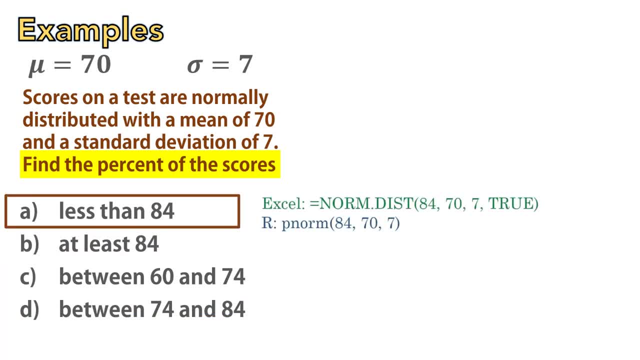 In A we want the probability that the score x is less than 84. So for x equals 84, the corresponding z-score is 84 minus 70 divided by 7. And that gives z equals 2 or 2.00.. 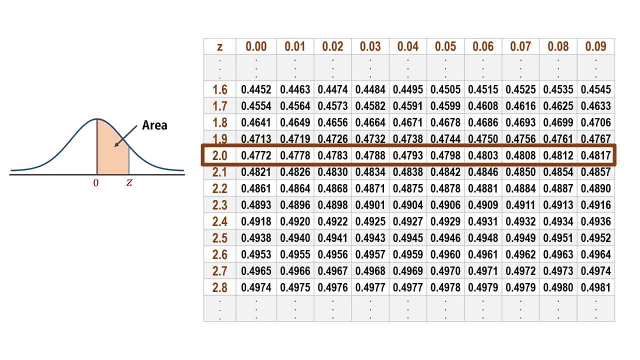 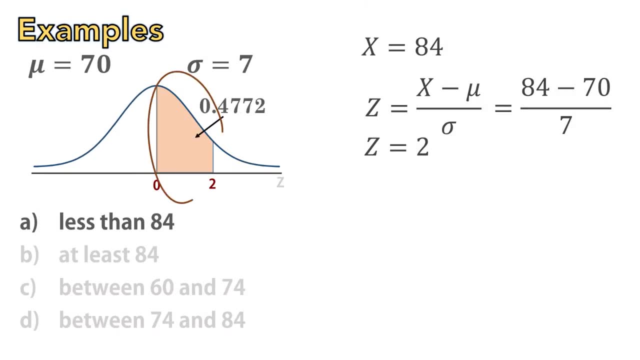 Now on the z-table, we look up z equals 2.0 or 2.10.. under 0.00 to obtain an area of 0.4772.. That is the area from z equals 0 to z equals 2 is 0.4772.. Therefore, this shaded area is the area we. 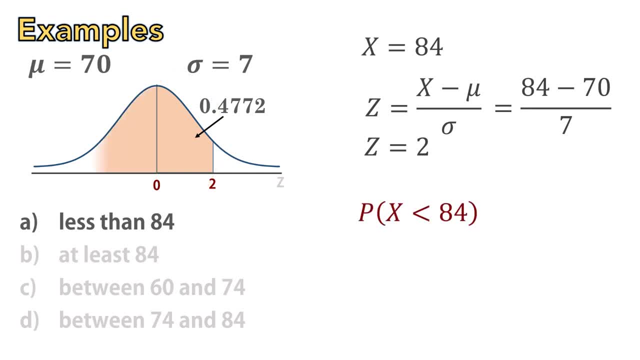 found in the table. However, the probability that x is less than 84 is the probability that z is less than 2, which is the total area below z equals 2.. Since the area to the left of the center here is 0.5,, the total area below z equals. 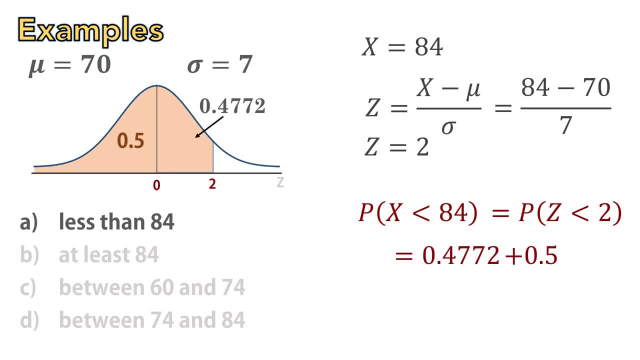 2 is 0.4772 plus 0.5, which gives 0.9772 or 97.72% For part. we want the probability that x is at least 84.. Recall that the normal distribution is a continuous distribution. 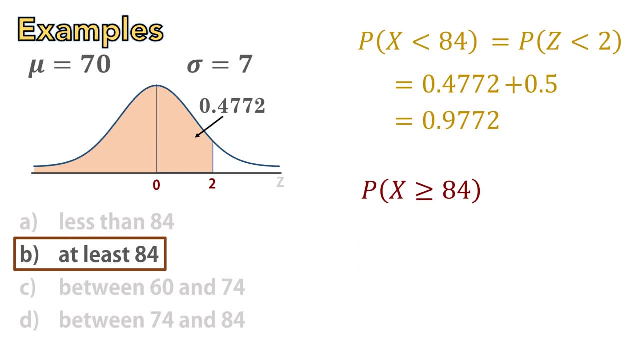 so there is no distinction between x is at least 84 and x is greater than 84. We apply the same approach in both cases. Also, recall from a previous calculation that when x equals 84, z equals 2.. So we will be correct in saying that the probability that 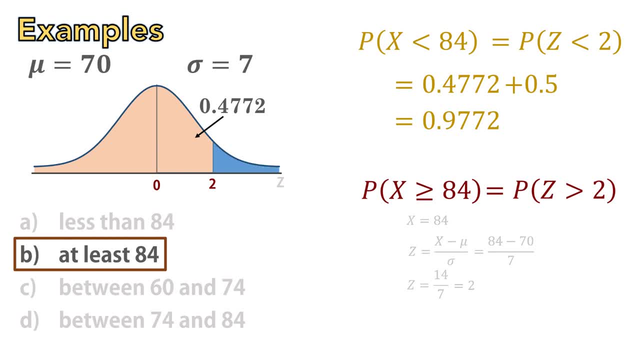 x is greater or equal to 84 is equal to probability that z is greater than 2.. And one way to find this greater than probability is to subtract the less than probability from 1.. If we don't have the less than area, since 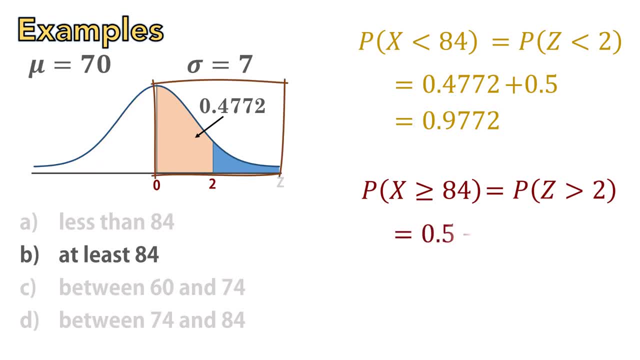 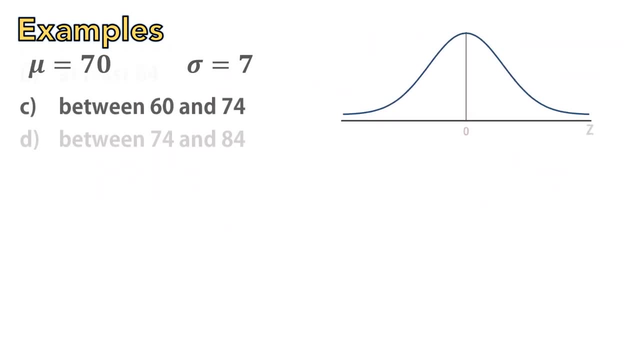 the area above the mean is 0.5, we can do 0.5 minus 2. So we obtain: x is 0.4772.. In part we want the probability that x is between 60 and 74.. For x equals 60,. 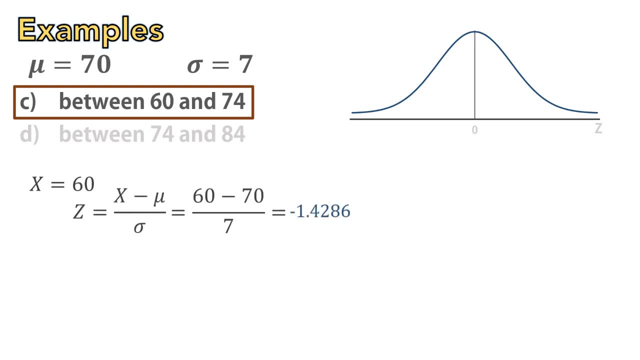 z equals negative 1.4286, which becomes negative 1.430 when rounded to two decimal places. We have to ensure we round correctly to two decimal places if we are using the table Also for x equals 74,. the standard normal score is 0.57.. Recall that we do not have 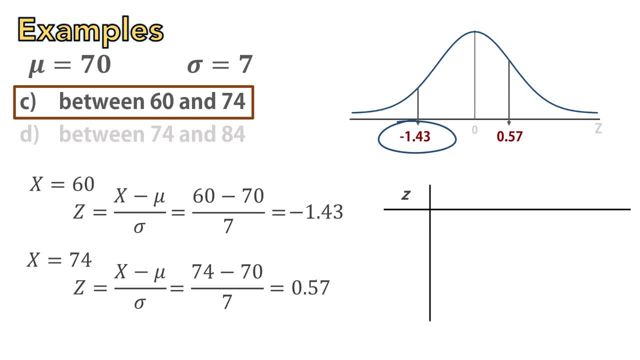 the negative z values on the mean to z table. Therefore, for z equals negative 1.43, we will look up 1.4 under 0.03, which gives 0.4236, is the same area from 0 to negative 1.43. because of symmetry. 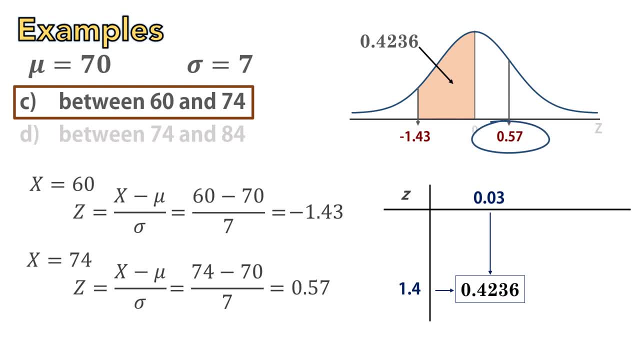 Similarly, for z equals 0.57,, we look up 0.5 under 0.07, and that gives 0.2157.. Thus the probability of obtaining a score between 60 and 74 is found by adding these. 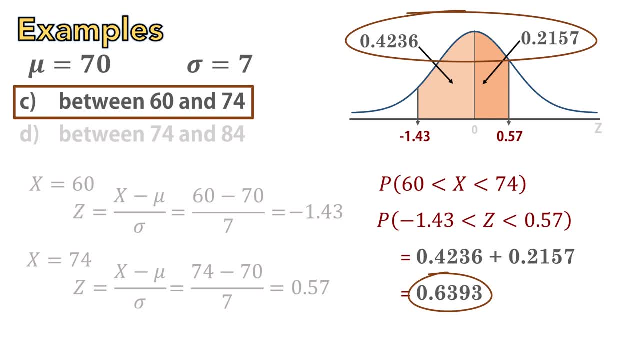 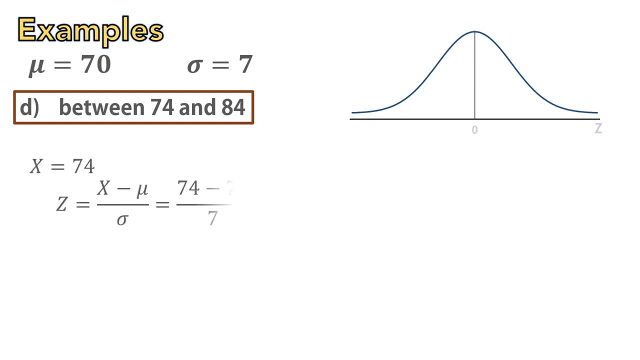 two areas, and that gives 0.6393.. Finally, we find the probability of a score lying between 74 and 84. When x is 74, z is 0.57, and when x is 84, the z value is 2..